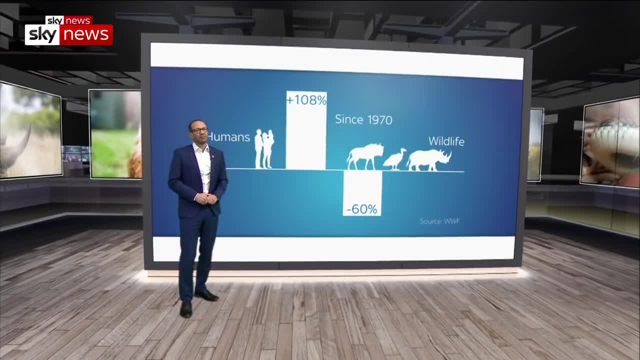 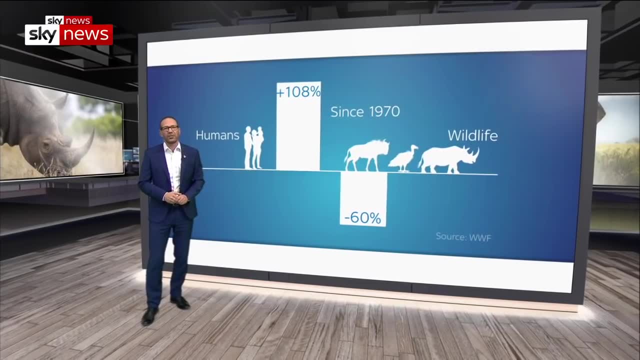 There are now 7.7 billion people on the planet. That's more than twice as many as in 1970.. Over the same time, wildlife populations have decreased by an average of 60%. Our runaway consumption of energy, land and water is killing nature. 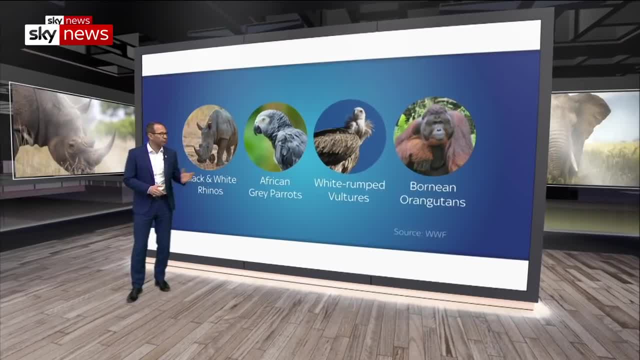 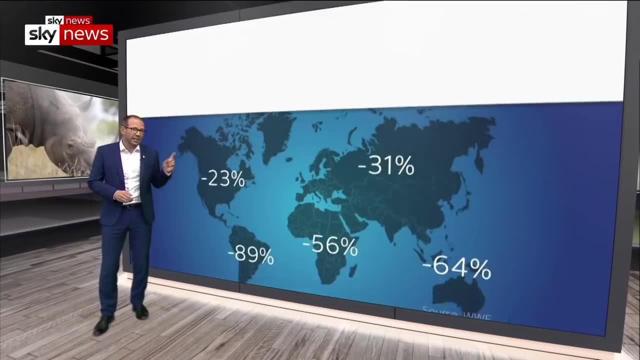 According to WWF's Living Planet report, species such as rhinos, African grey parrots, white rump vultures and born-in orangutans are all in decline. Latin America and the Caribbean, home to the jaguar and the giant ant eater, are worst. 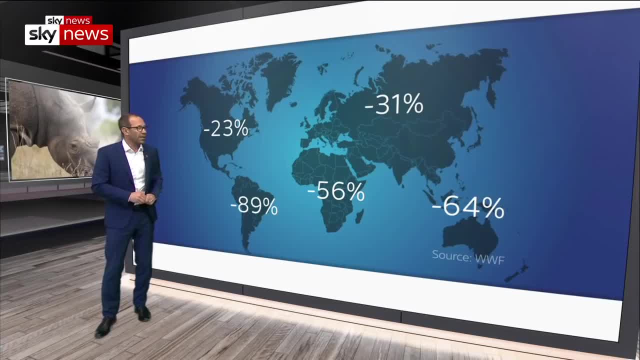 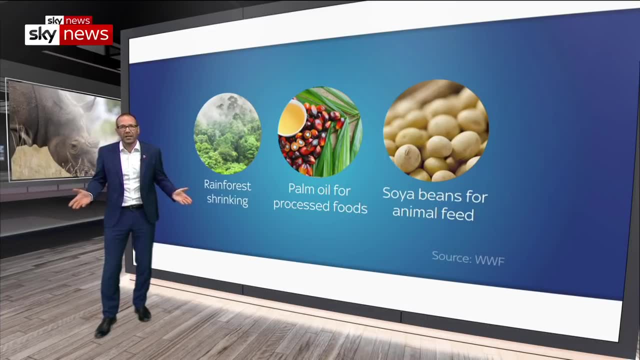 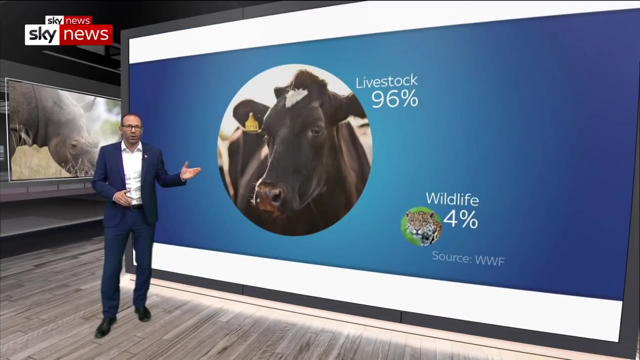 affected, with populations of monitored species down by 89%. Their habitat, the tropical forest, is shrinking. Trees are being replaced by farmland palm oil for processed foods and soya beans for animal feed. And take a look at this. Livestock is replacing wildlife Of all the mammals in the world. 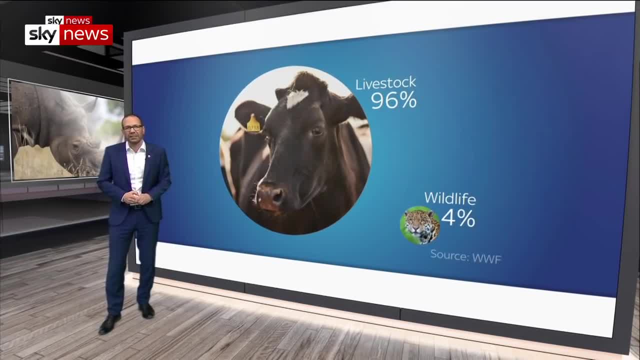 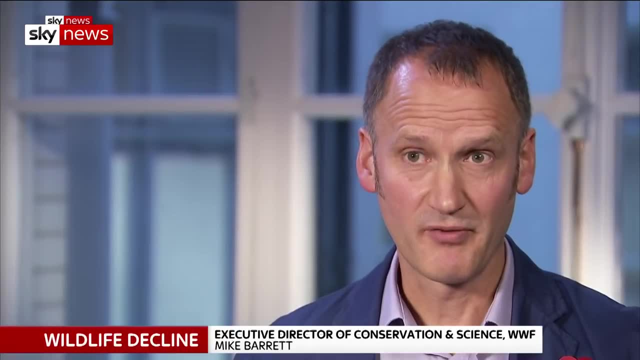 apart from us, 96% are cattle, sheep and pigs. Just 4% are wild species. The loss of habitat in one part of the world, as well as being driven by what happens in another part of the world, also impacts what happens in those parts of the world. So for 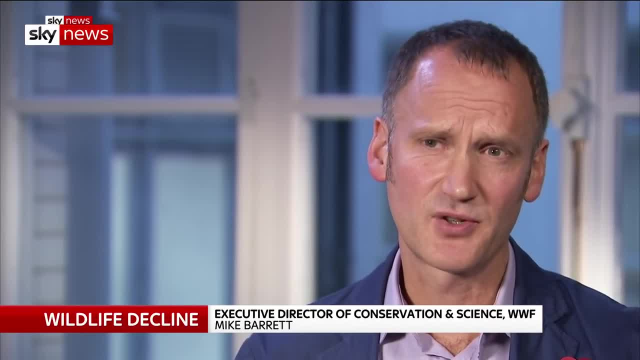 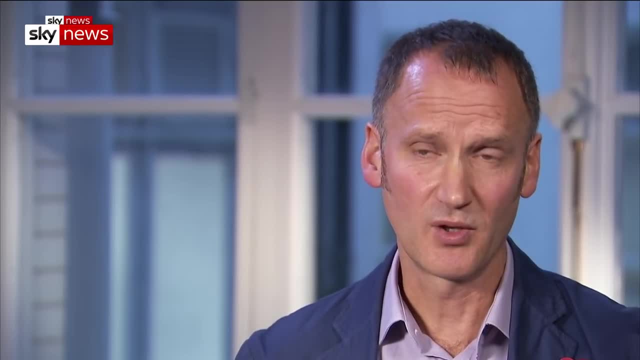 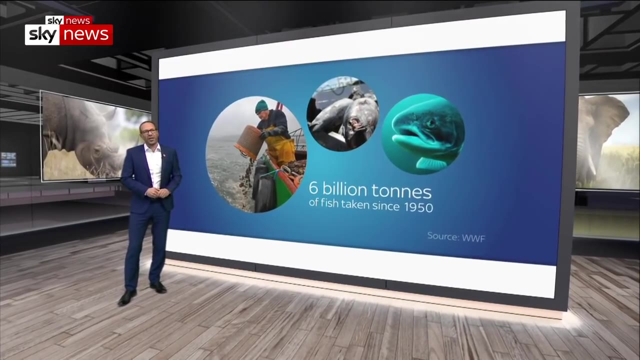 example, losing the Amazon rainforest would be absolutely catastrophic from the point of view of tackling climate change, So it matters to all of us that we should make sure that these key parts of the world are not damaged any further. The oceans are in decline, too: 6 billion tonnes of fish, shellfish and other creatures have 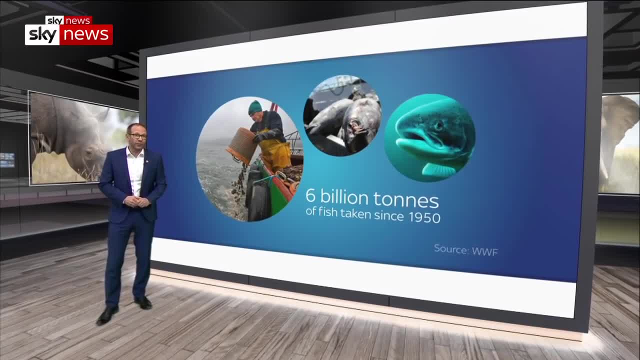 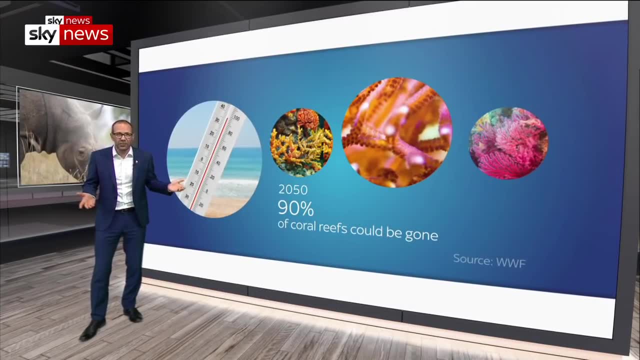 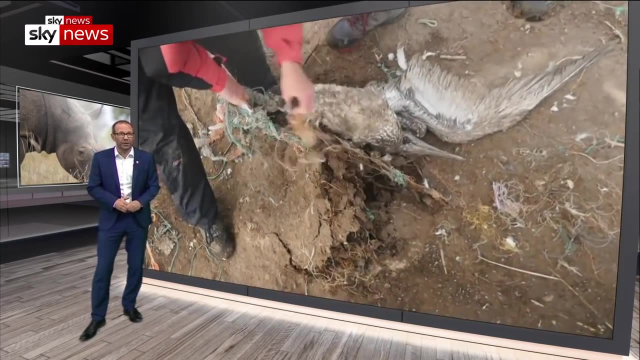 been taken from the seas since 1950.. With industrial fishing pushing some populations to collapse, warming seas driven by climate change are killing coral. By mid-century, 90% of reefs could be gone And, as we've highlighted with the Sky Ocean Rescue campaign, plastic is being eaten by. 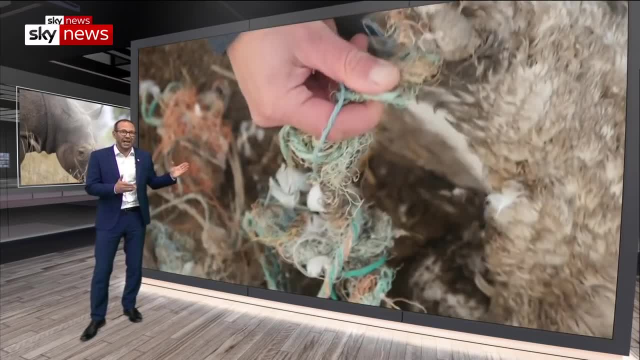 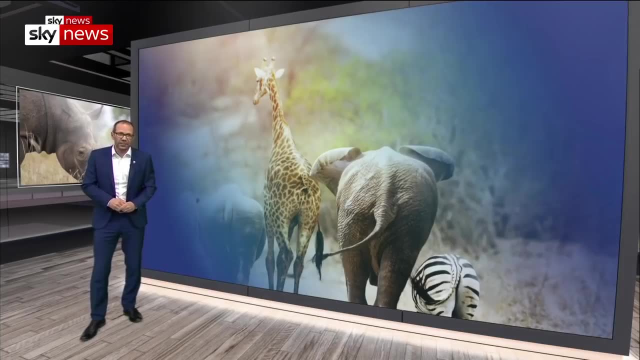 fish, turtles and whales And, as I've found off the Welsh coast, gannets are even raising their chicks in nests of discarded fishing nets, with tragic consequences. In two years' time, nations will gather for the United Nations Convention on Biological. 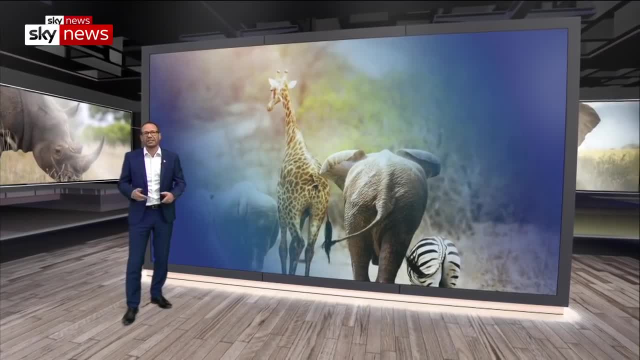 Diversity. WWF says habitats need protecting and the economy made more sustainable to reverse the decline in wildlife.